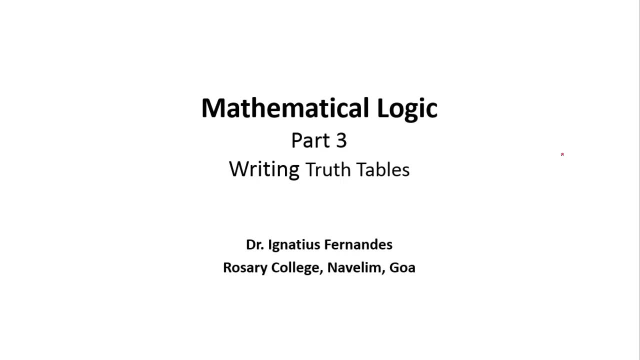 Welcome back to module 3 of this unit 1 of this mathematical project, And we will be talking about how to write down a truth table for a compound state in this module. Now, before you start with this module, you have to make sure that you know the truth tables for the five connectives that we talked about in the previous two modules. 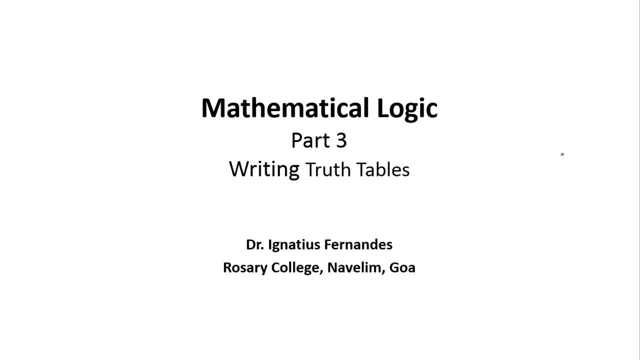 That is, OR AND NOT CONDITIONAL and BICONDITIONAL, Because to write down the truth table for any compound statement, we will be using these five basic connectives. They are truth tables in writing, the truth values. Now let us say I want to write down the truth table for this compound statement. 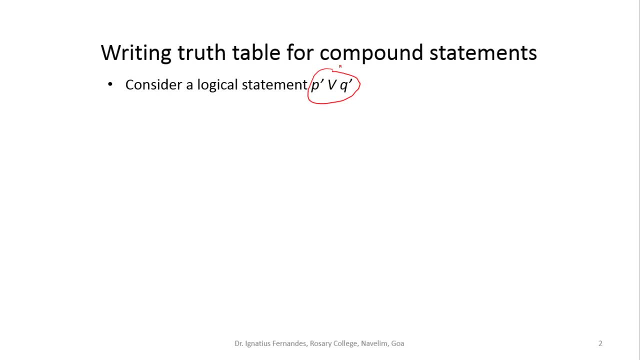 That is P, NOT P, or NOT P, That is P bar OR Q bar. So we want to write down: So this is a compound statement which involves two simple statements, P and Q, And then it is connected by two connectives: One is OR and the other one is NOT. that is involved here. 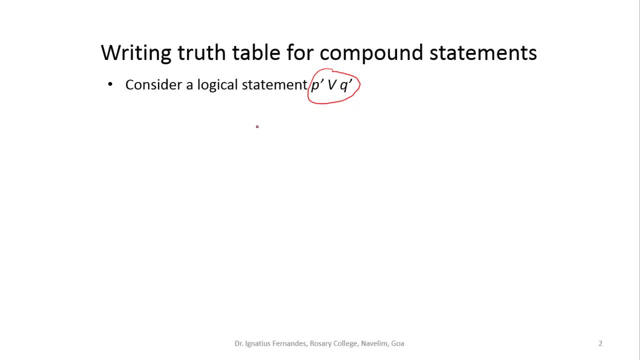 So this statement is symbolic form of some statement which has been put into a notation form, like this: This is what we know when we write down a statement In notation form like this, And let us say: I want to write down the truth table for this. 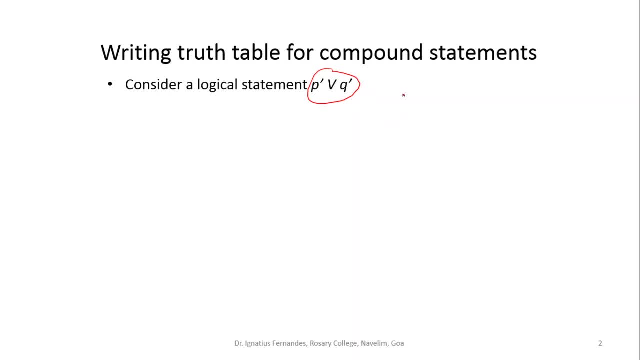 So, to write down the truth tables, we break it down into simple statements: There is P here, There is Q here, Then there is P bar here, There is Q bar here, And then finally we have P bar or Q bar. So to write down the truth table, what we do is we go in step by step, depending on the simple statements that I have written. 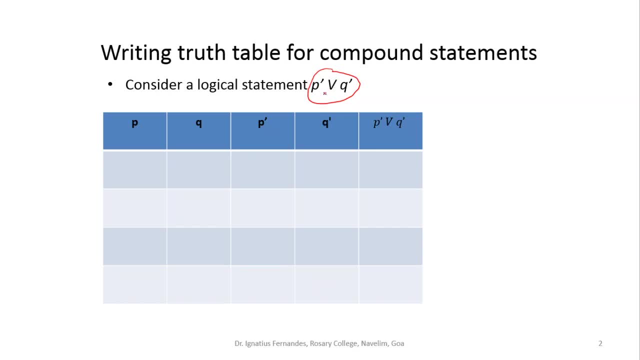 There are two simple statements that are involved here. There are two simple statements that are involved here- P and Q- So I have P and Q. There is P bar that is involved here, So I write down P bar. There is Q bar that is involved here. 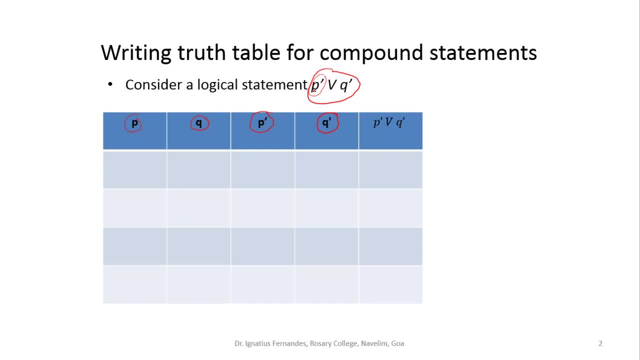 So I write down Q bar And finally, after I know what is P bar and Q bar, I can write down P bar or Q bar. Now this is our statement that we are having, And we will need the truth values of this statement. Now, P and Q are two statements. 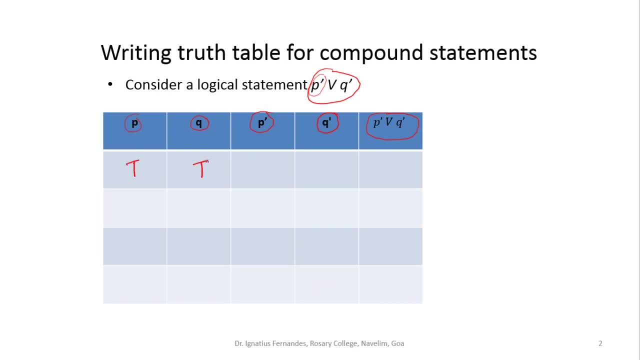 So, as we know, they both can take values T and T, T, F, F, T and F F. Either both can be true or both can be false, or one of them is true and the other one is false. Now to write down the truth values, you have to make sure that you know the truth tables of not because we are using not here. 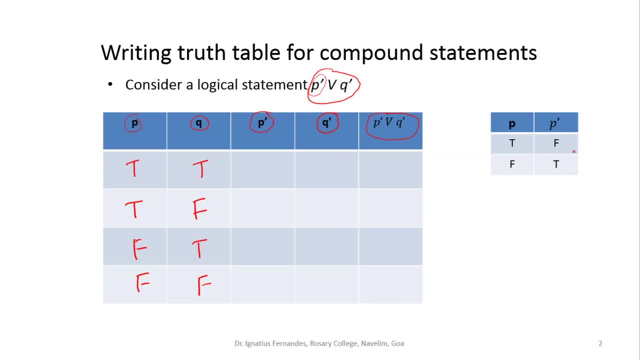 So this is the truth table of, not that I have highlighted here, But then in your mind. you should always know this truth tables. If not, then revise those truth tables first and then come back to this example. The same way, I will also name the truth table for or. 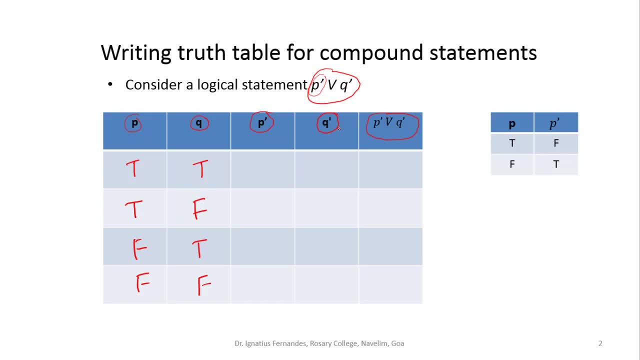 So I should have in my mind the truth table of, or The truth values in case of. we have a or connecting, And this is the truth table that we wrote earlier for or. So now coming back to this table, Now for P, I am writing, not P. 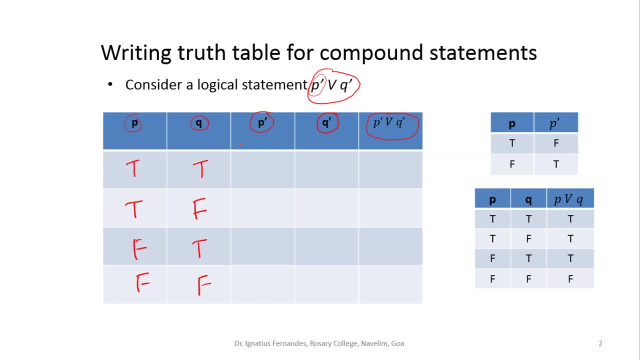 So I have to write down the opposite of P. So if P is true, I know that not P is false. Here P is true. so not P is false Here P is false. so opposite of that is true. P is false here. so opposite of that is false. 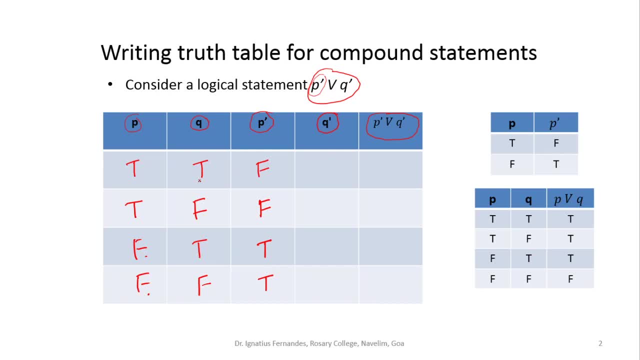 The same way I write down, not Q. So if Q is true, not Q is going to be false. If Q is false, not Q is going to be true, opposite of that. Now, Q is true, so opposite of that is false. Q is false, so opposite of that is true. 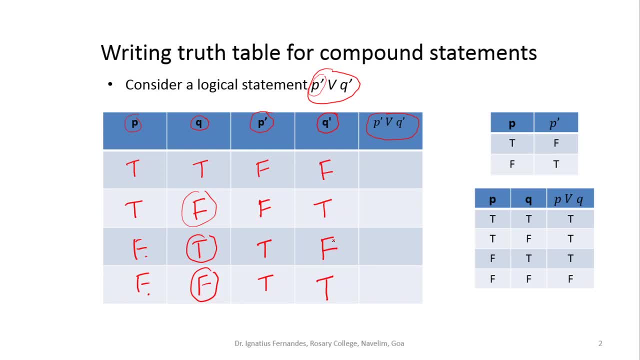 So these are the not values. After I have got these columns, now I go to the final column. So I write P bar or Q bar. So I have P bar here, I have Q bar here. Now I use, or So I should be using, or for these two columns here. 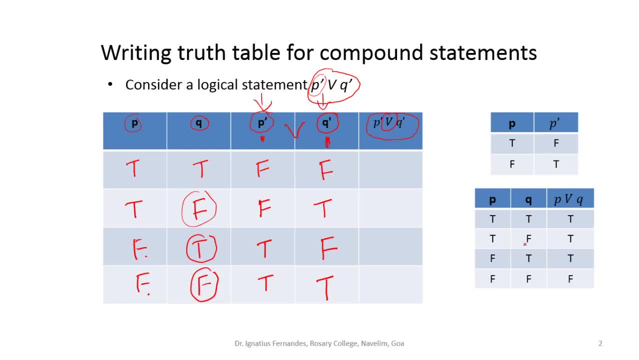 This column and this column. Now for that I go back to. or truth table, This was the table for, or I know that, or is true when at least one of them is true. Otherwise it is false. So for F and F in or case. 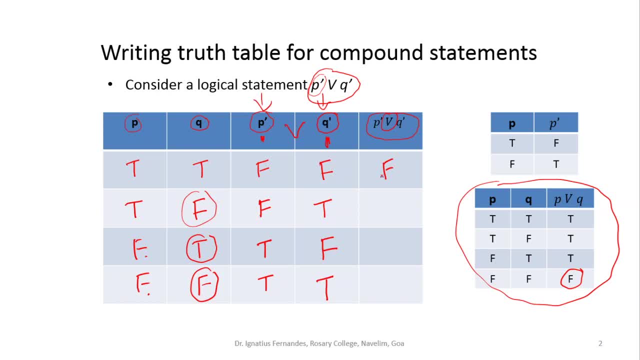 F and F it is F When both are false or is false. One of them is true. or is true. For F and T it is T. So I wrote T here For T and F. T and F is T, For T and T it is T. 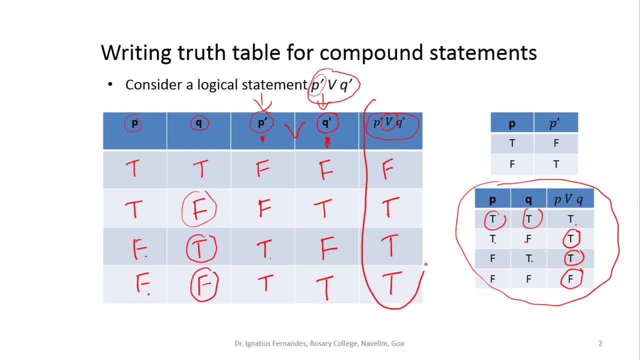 So it is T. So this is the truth table, or truth values, of this compound statement that we were trying to write down. So this is how you should be writing the truth table for any compound statement: Write it down into simple statements Depending on how many, what parameters are involved, and then come to the final column. 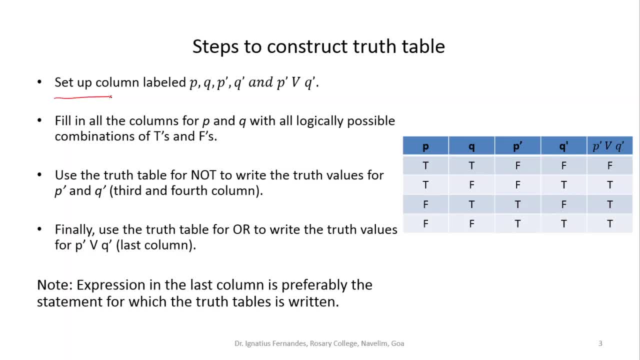 So basically, the steps to construct the truth table is: you first set up the columns, like how we did for P, Q, P bar, Q bar, And finally the statement that is under concentration. Then we write down the values for P and Q. 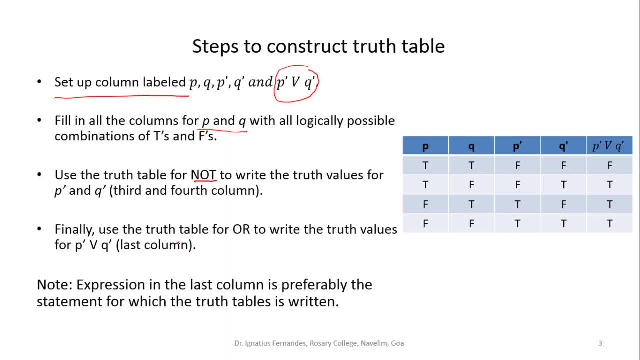 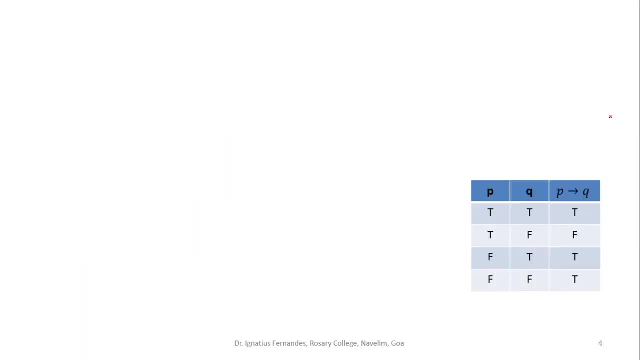 Then we write down the truth table for not And wrote down the values for P bar and Q bar, And then, finally, we wrote down the truth values for P bar or Q bar. So in this example, this is how we pick it up. Let us say you have another example. 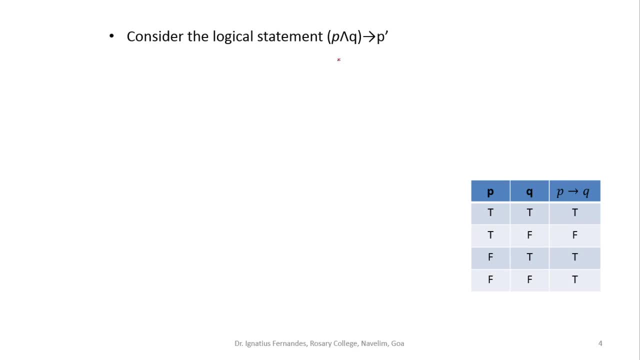 You want to write down the truth table for this compound statement That is P and Q implies P, bar. So Again the same way. there are two connectives that are involved here. One is AND and other one is conditional. So you should remember what are the truth tables for AND and what is the truth table for conditional. 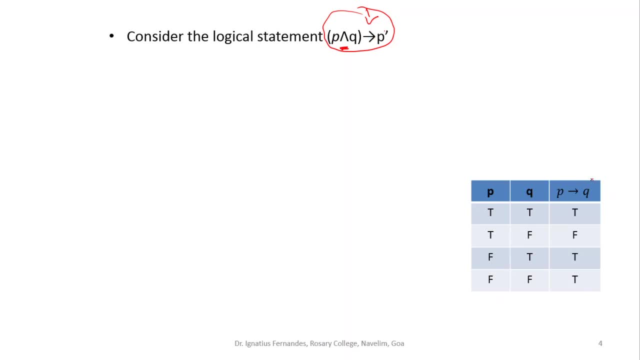 Now conditional truth table is already here to recall. So to write down the truth table for this, We break it down again. So there is P involved, There is Q involved. So first column will be P and Q, Then we will find out what is P and Q. 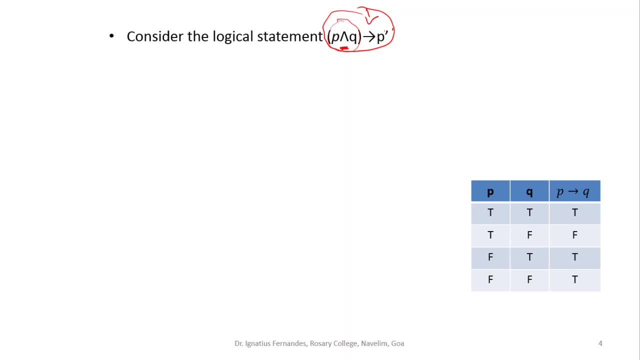 We need P bar, So we will find out P bar, And once we have P and Q and P bar, Then we will use conditional for this statement. So this is how I write it down. So I have P and Q, So I wrote P and Q. 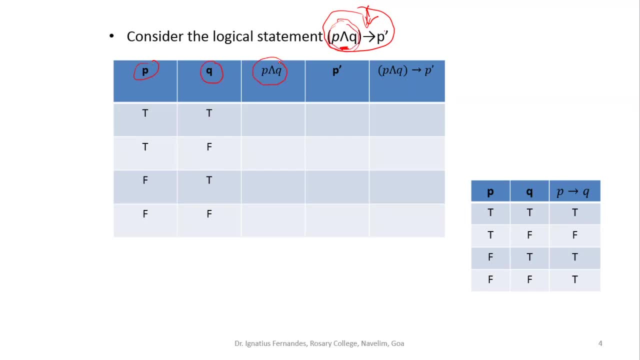 Then I wrote P and Q. I need P and Q, I need P bar also. So I made a column for P bar. And finally to this statements between it Now, P and Q. we already know it can take the values T, T, T, F, F, T and F, F. 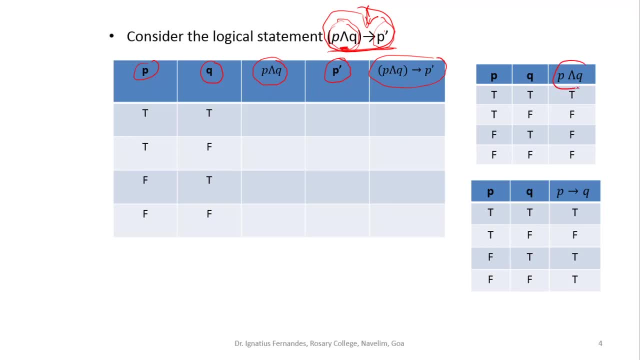 So recall the truth table for AND. This was the truth table for AND, And we know that AND is true only when both of P and Q are true. If at least one of them is false, then Q is false. Okay, So for P and T it is T. 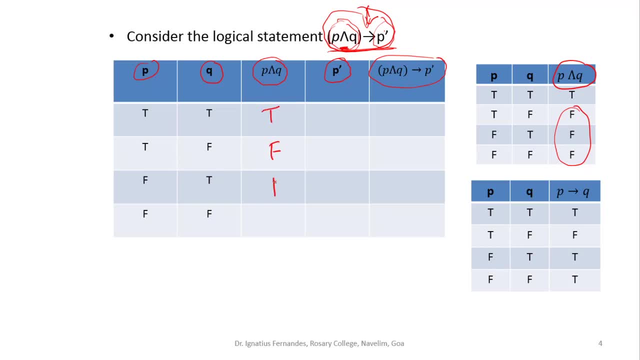 For T and F. it is F For F and T. it is F For F and F it is F. I am using AND in truth table. So this is why you need to remember all those five basic truth tables. We write P bar now. 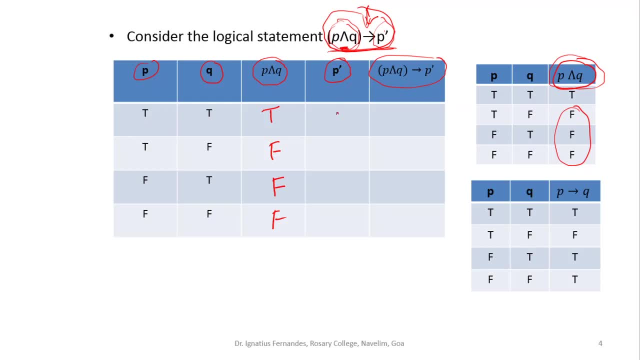 So it is the opposite negation. So if P is true, this is false. If P is true, this is false. P bar is false. If P is false, P bar is true. If P is false, P bar is true. So I have got T and Q. 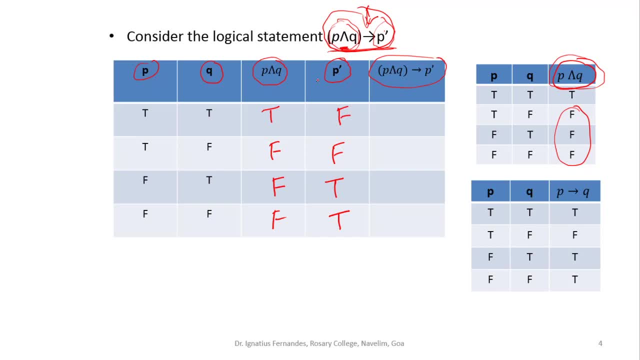 I have got P bar, Now I use conditional, So I use conditional for this. Now, conditional truth table is this: For T and T it is T, T and F it is F. For F and T and F and F it is T. 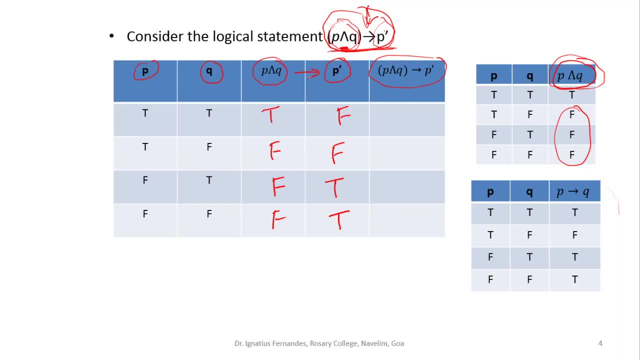 So this you should know. So I use conditional truth table for this column and this column For T and F. For T and F it is T, For T and F it is F. So I write F here For F and F it is T. 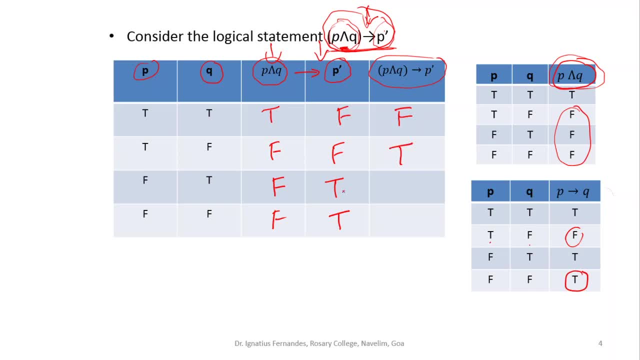 So I wrote: I write T here For F and T. it is T. So I write T here And for F and T again it is T. So these are the truth values for this statement And this we will say is the truth table for this statement that we are going to write. 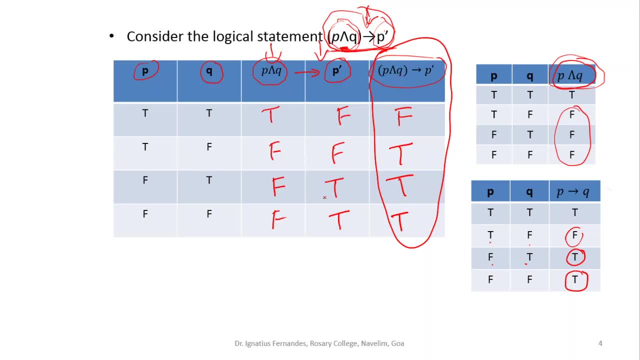 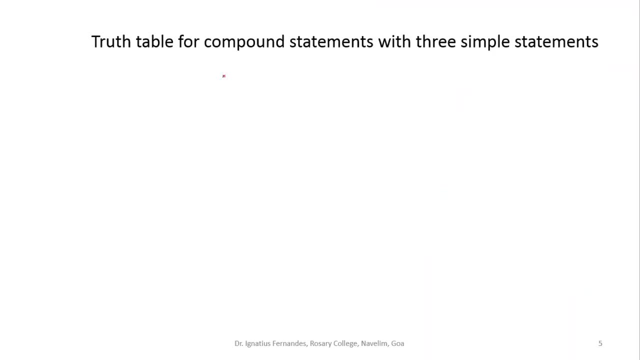 And this we will say is the truth table for this statement that we are going to write. Now, these were examples wherein we consider two simple statements: P and Q. Now, these were examples wherein we consider two simple statements- P and Q. Let us say I have three simple statements involved. 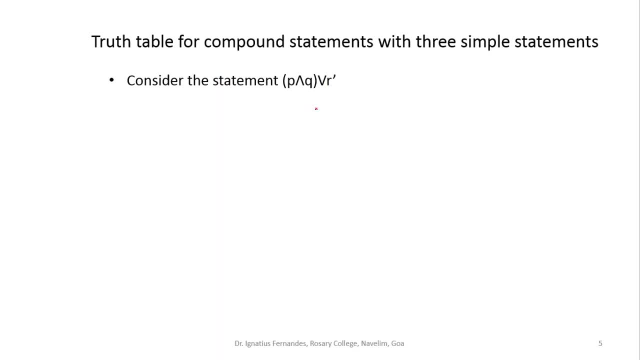 P, Q and R. So I want to write down the truth table for this particular component statement, which involves three simple statements: P, Q, R. Again, the procedure will remain the same, Except that earlier we had only two columns starting, columns P and Q. 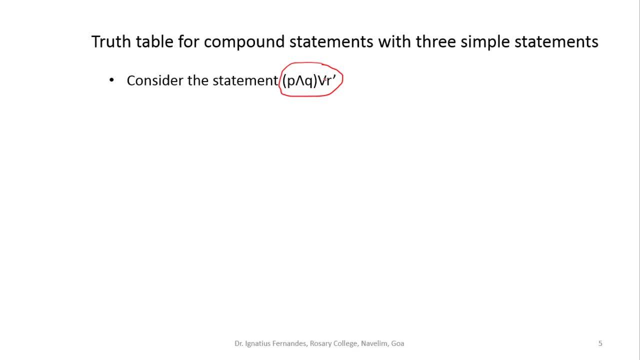 Now we will have three starting columns: P, Q and R. So again we break it down. So we will need P and Q, a column for P and Q, We will need a column for R bar, And once we have this, then we will find out P and Q or R bar. 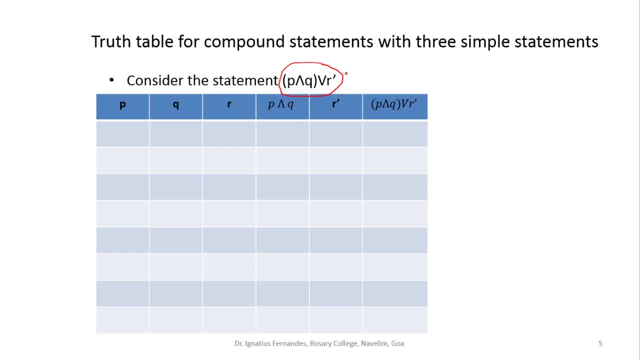 So this is how you will form the table. So I need P Q R. So there are three statements: P Q R. I need P and Q, So I made a column for P and Q. There is R bar here. 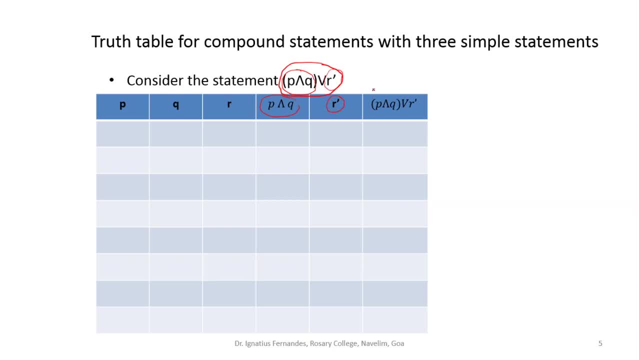 So I made a column for R bar. And finally, the component statement that I am looking at Now. P Q R. there are three statements here. Each one of them can be either true or false, So accordingly, I will have T T T. 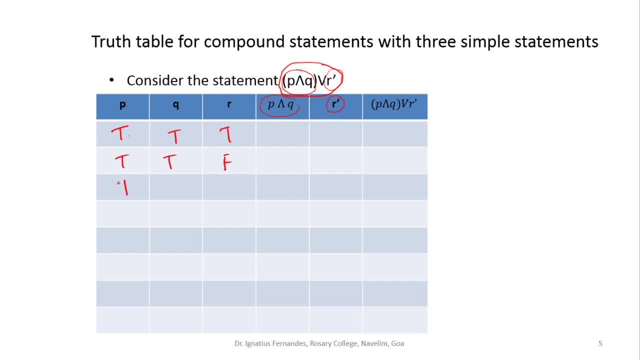 T, T, F, T, F, T, T, F, F, F, T, T, F, T, F, F, F, T And F, F and F. There are the eight combinations of the truth values for three statements: P, Q, R. 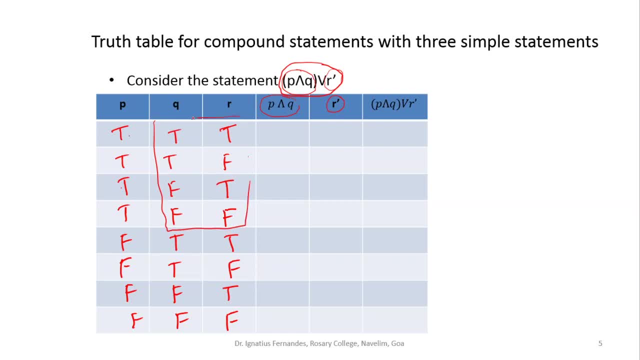 What I have done is now- this is one part that you already know- You have been writing for two cases, two statement cases T T, T, F, F, T and F? F, When there were P and Q. 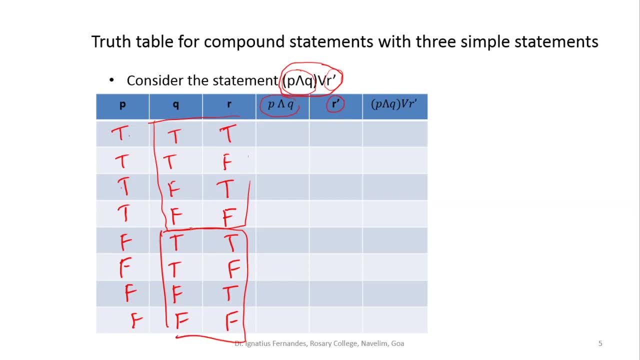 So I have repeated the same set again here, This whole part. this part I have copy pasted here, One set with all T's and the other set with all F's. Same way you can write down the truth values, for if there are four statements. 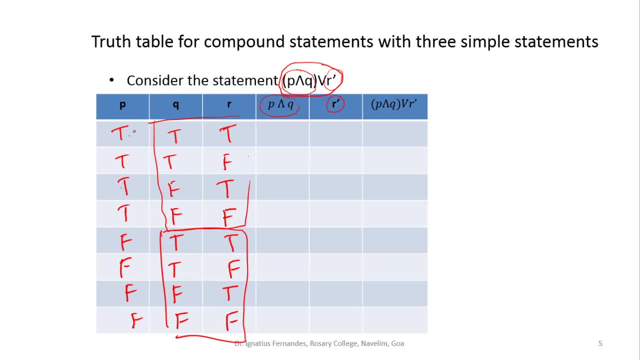 Now, in case of three statements, simple statement, there are eight rows. In case of four statements, it will be sixteen rows, And so on. So I need the truth table for AND. There is, AND that is involved here. So I recall in my mind the truth table for AND. 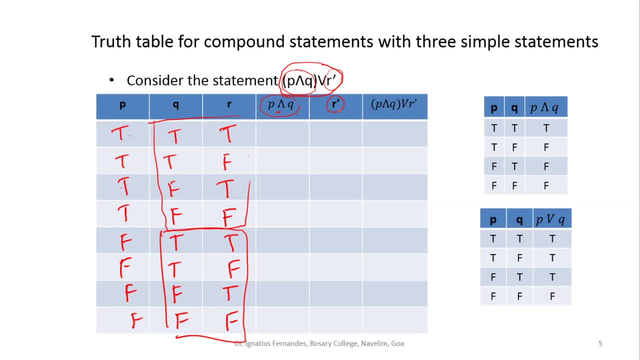 And there is NOT that is involved here. So, and then there is OR that is involved here. So I have to recall the truth table for OR And there is AND There is NOT also involved here. but NOT is very simple. So I start writing the truth values: 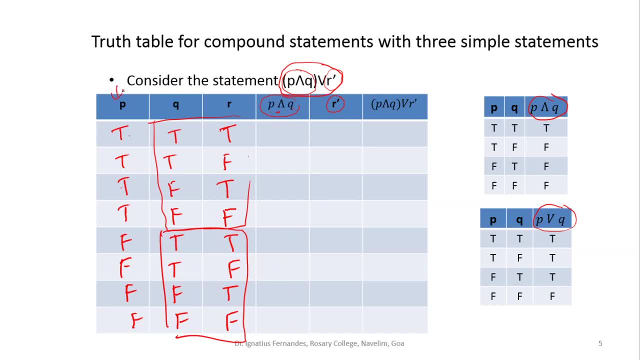 So I am writing P and Q, So I have to look at P, I have to look at Q And start using AND truth table. So for T and T, For T and T, it is T, For T and T, it is T. 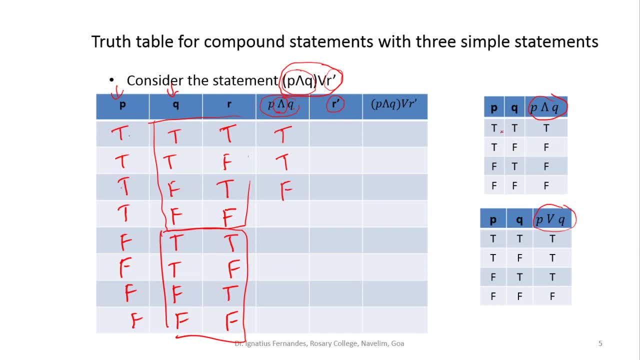 For T and F it is F. So I am looking at T and T, I am looking at, AND. So for T and T it is T, For T and F it is F. So that is how I have got F here. For T and F it is F. 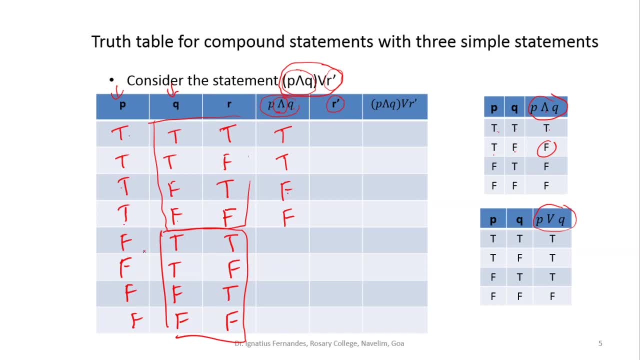 Now, there is at least one F in all this, And I know that. AND is false when at least one of them is false. So all these are going to be false. This is false. F and T is false. F and T is false. 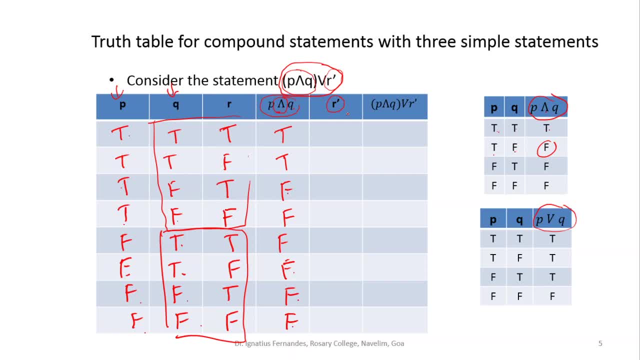 F and F is F. F and F is F. Next I write down the column for R bar. Now, R bar is the opposite of R. So if R is T, its opposite is F. If it is F, it is T, For T, it will be F. 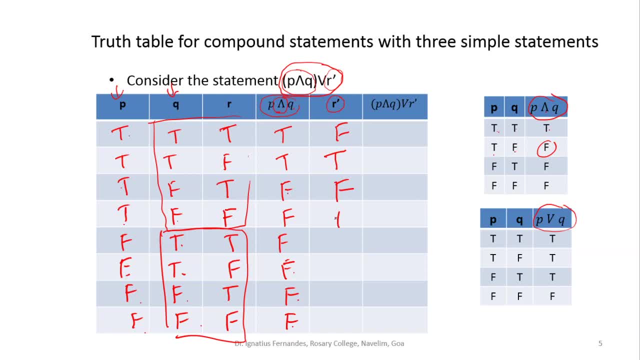